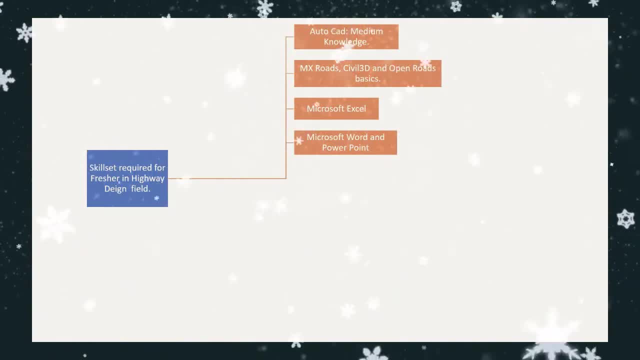 things that It's not required for a civil engineer. This weren't enough or fine, because when you grow means uh, from small position to higher level, from engineer to senior engineering, and then what to say? Principal engineer notion person could get that二. have three limits: Either. So the PPT, knowledge and the PPT should be available, but very few were not. Oh, one may have a choice, but other ways are possible. Okay, Then the third base decision board has already been approved. that needs to be analyzed in a Bible. 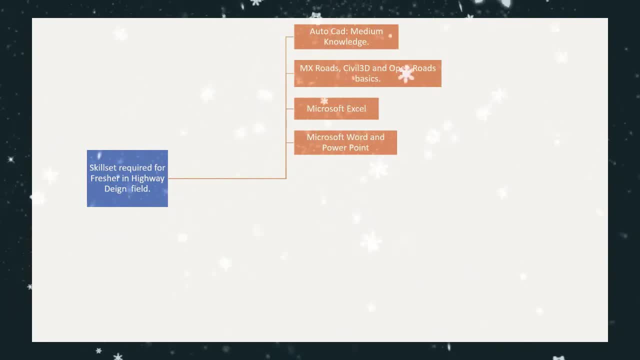 movedani foremark averly goes to actually in it. So this that needs to be analyzed, All those things. so many functions are there that I should be there. Okay, Then, word and ppt. knowledge and ppt should be prepared by our own, ourselves to impact the client. okay, so good. 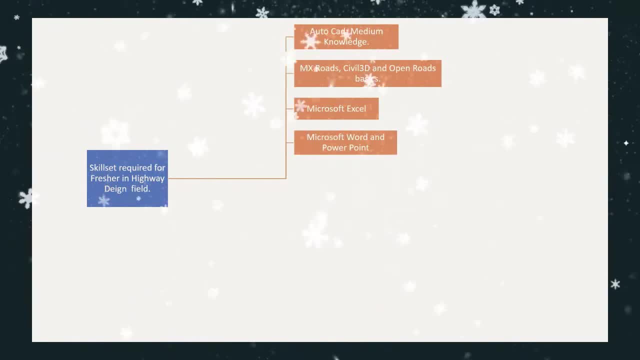 skills, make a good what to say, good projects and then good revenue and everything will be a positive manner. so, powerpoint and word, word formatting, all those things you need to aware. then google earth. google earth is very, very important, especially for doing the bypass options. uh, in highway design. yeah, in google earth, normal basics is enough. okay, then important. 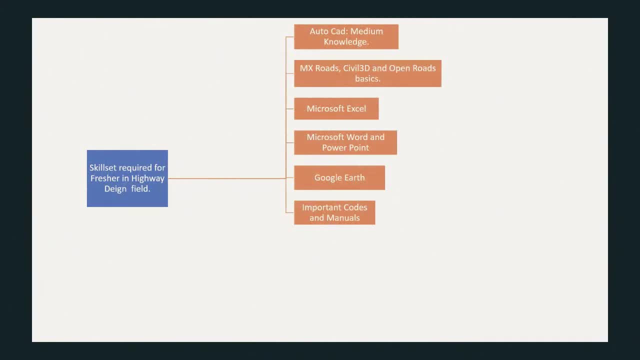 codes and manuals means like irc codes and dmrb codes, just simple basics is enough. if you remember the code name is: that is also very good. okay then for four lane: what is the code on flexible payment? what is the code that? that also a very good, and have a brief idea. that's it then. 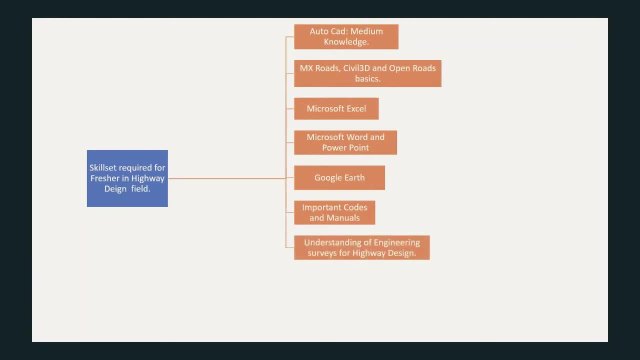 go to the engineering service. what type of engineering service is required for the highway design? that type of means road inventory and what to say visual payment condition survey? and so many surveys are there that they use to teach in a institute itself. some basic idea, if you read any. 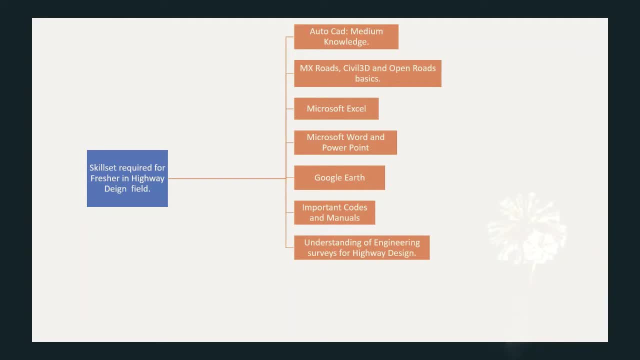 any. what to say? uh, just a book and kadi ali book, you will get a idea, basic idea: reconnaissance, okay, all those things. and then payment design basics- okay, just like what flick. what are the parameters required for flexible and rigid? that basic idea. and if you read the code perfectly, 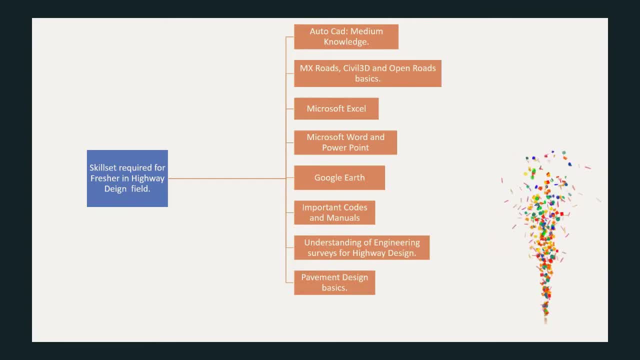 then you can understand it. but when you get into industry it will be a very different procedure. so but methodology will be the same. some may use excel, some may use some spss, but but the methodology is the same. but that's why i'm saying payment design basics. what are the 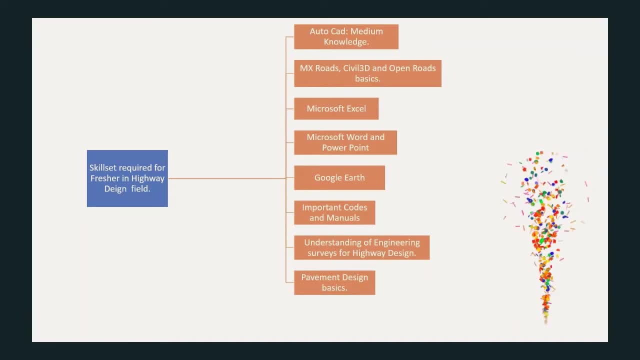 parameters required for flexible and rigid and what type of service required that under that overview is required. okay then traffic service. see this payment design basics is entirely dependent on the traffic service because, based on the traffic only will estimate the thicknesses, so how it is going to conduct normally in a mtech or btech the traffic service should be. 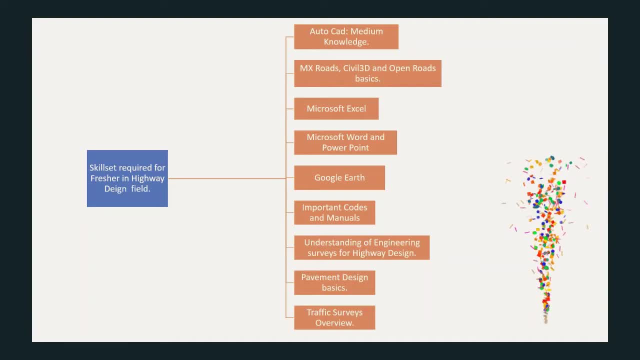 conducted by the students for any other reason, for research purpose or for consultancy- easy works, but so there must be idea, so no need to worry. but some analysis, data processing is there, how, how we need to do that. things should be aware. okay. so these are the important contents. 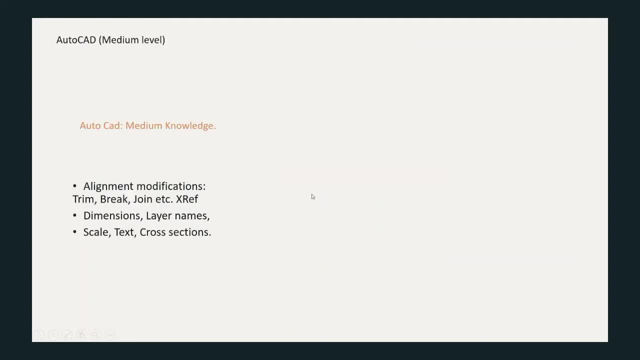 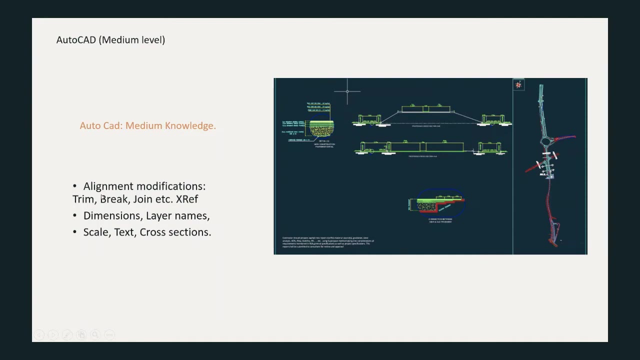 is required. okay, let's start. start one autocad. autocad medium level. that's what i said. medium knowledge is enough, no need of expert. so when you join in a highway industry as a fresher, okay, before joining, so you should be aware about this command trim. 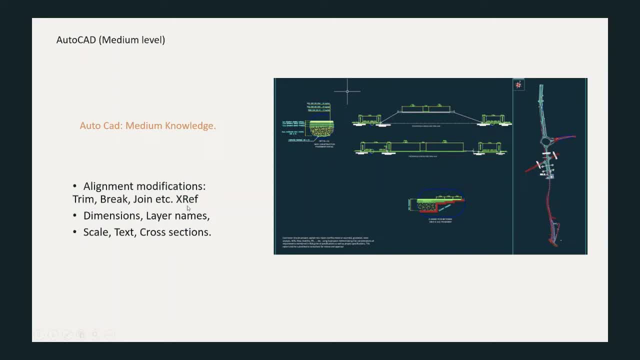 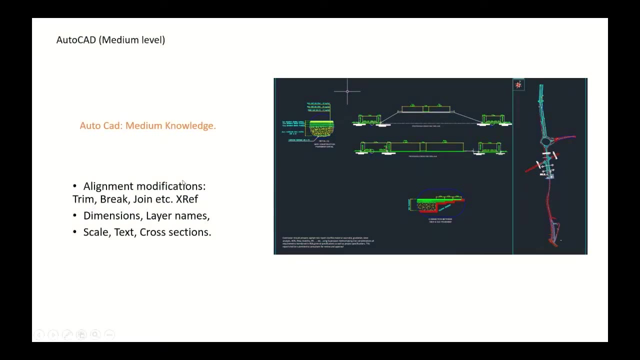 break command xrefs- how to attach xref images: okay, and how to prepare a cross section and some modifications in the line trimming and fillet: okay. those options should be aware. that will. that will give a good man's opinion about you. means he is having some good knowledge, means at least basic knowledge. is there no need to teach him. 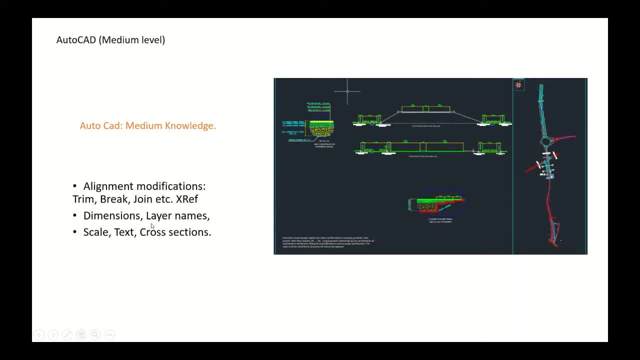 that comes from the manager and dimensions and the layer names. okay, after that, scaling text, annotation, cross sections, preparations, okay, these things you must be aware because there are so many sources to learn now youtube is there and linkedin learning is there and so many sources are there. 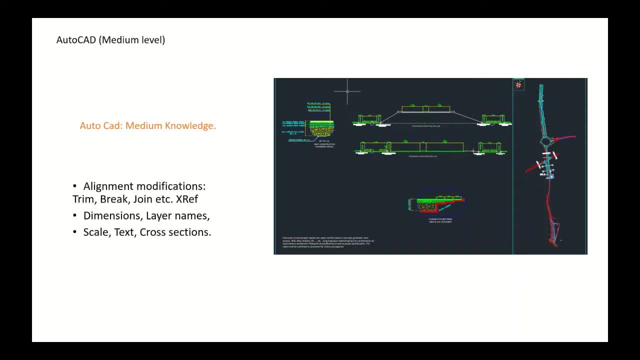 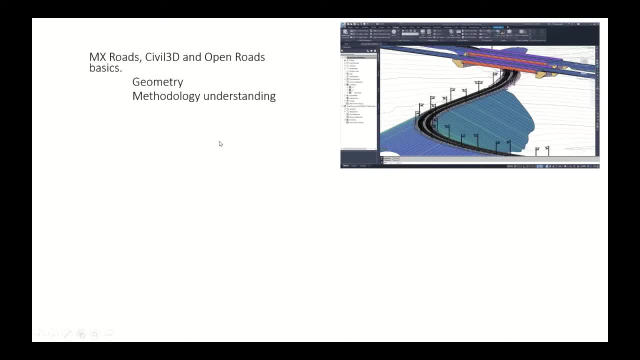 so please have a good knowledge on this autocad. okay then mx road civil theory and open road basics. okay, this is civil 3d, but in these things you just need a basic idea. what is the methodology to use? okay, and how the process will starts, how normally we will take a survey data and then 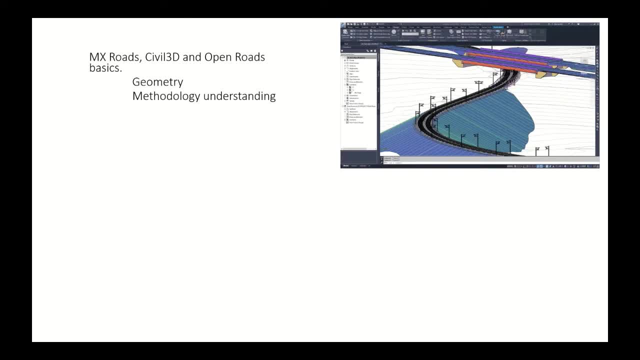 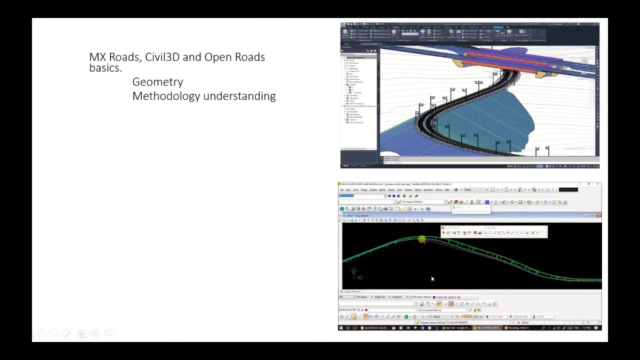 import it and then we will start the geometry, like that, the basic methodology you should understand, no need of in-depth knowledge, basic methodology is enough. okay, some important contents. okay, that's what i'm saying. so then this is mx road. mx road is different, like string based, and civil 3d is. 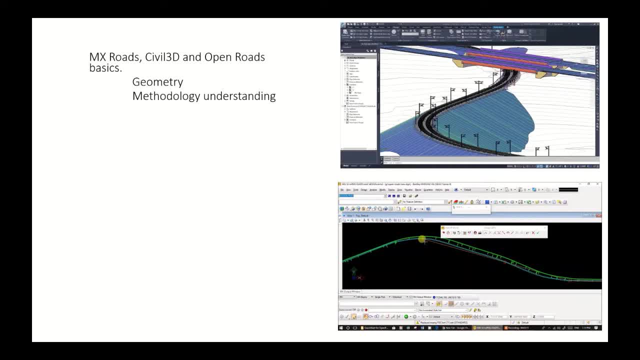 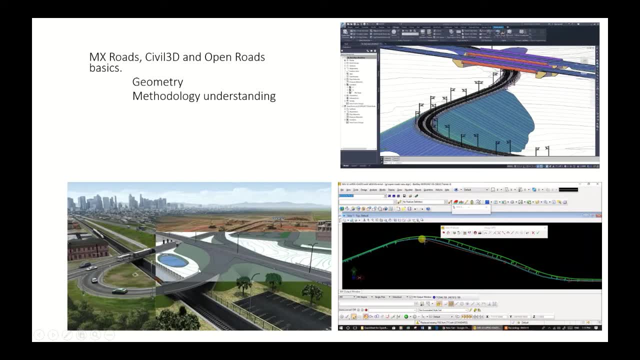 a template. template based and then open route is also same template based. here it will call assembly and we will call a template. that's a basic difference. but both are similar tool. these are tool based. this is under. this is a string based concept. okay, that that you should understand. 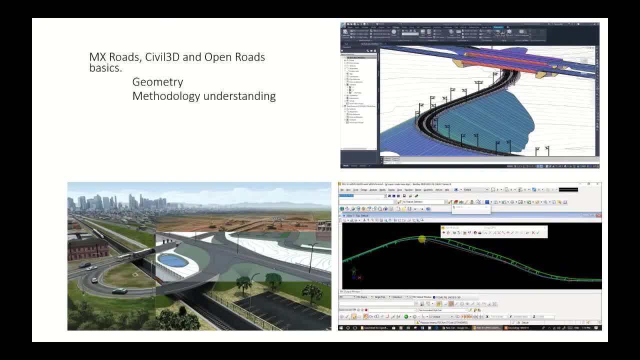 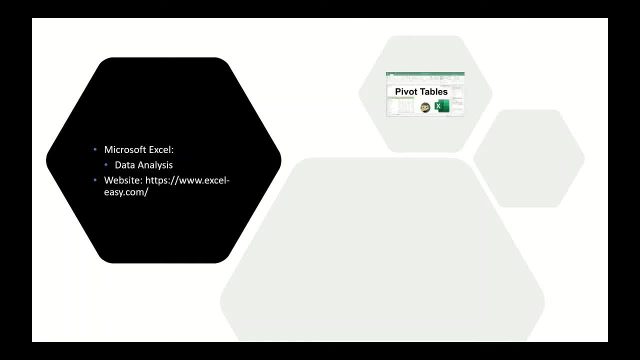 normally in interview somebody means the interviewer may ask okay, and then so private instagram, sorry, public smi is there, although it is a small one, uh, but to安, thats very nice idea and it will understand you as a public name you must be able to remember in. 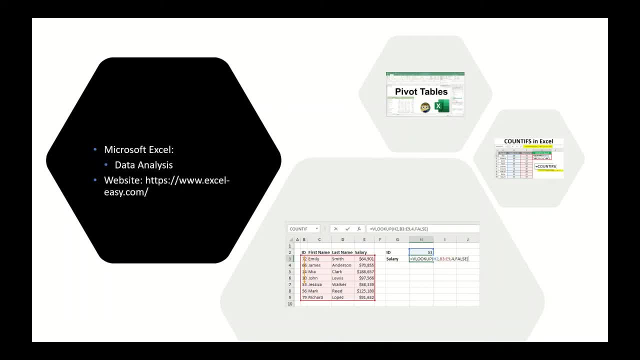 you must be able to know yourself right from the verdad me. we're not sure how to lead on the internet. you're entering into the instagram to text kind of definite in your name. you should have that kind of passed interview. so you're doing different on the internet. it's also not in existent form. it's in there in the userDR, which here maybe not necessary. listen, you talk in different language, not necessary? fine, get out of the actual language and try to do everything in all of the structures in the list, from terms of body count and all this things. 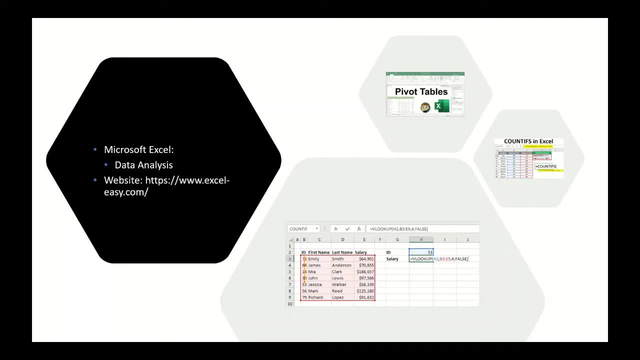 um, remember sometimes what happens if they give us some work. normally take so much time, but if you think and write some useful function, okay, then you can reduce the manpower. that will create a good impression to the manager. okay, that's what happened one or two times with my 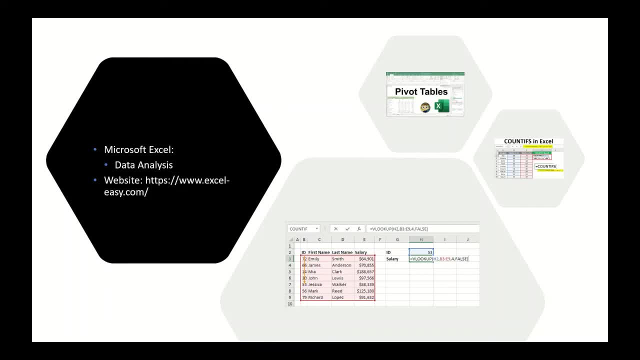 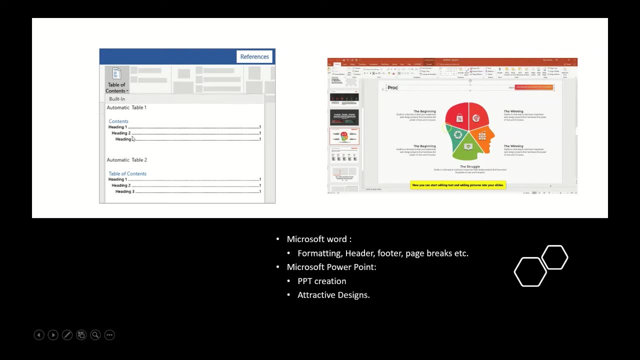 friends and myself also okay. so that's why i'm saying: some good functions you should learn before starting a career. okay, and then what? that's what i said in the beginning: in the world formatting. formatting is compulsory because nowadays executives are there in each company, but sometimes what happens? 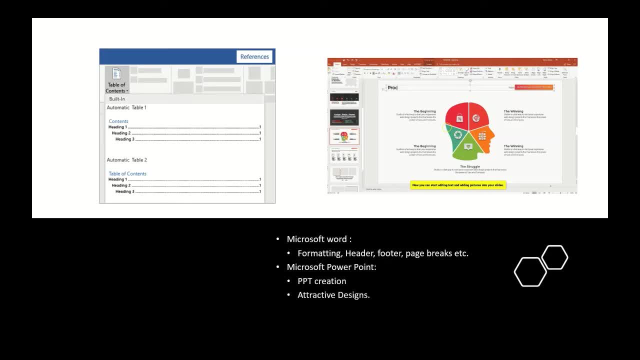 to the unavailability of the sources. uh, you have to do the formatting. so good, formatting report is a better, gives a better impression. okay, so formatting is required. and text aligning and tables adjustment: okay, that should come automatically when you do seriously on a project, mtech project- okay, so that's what. and then powerpoint powerpoint skills. 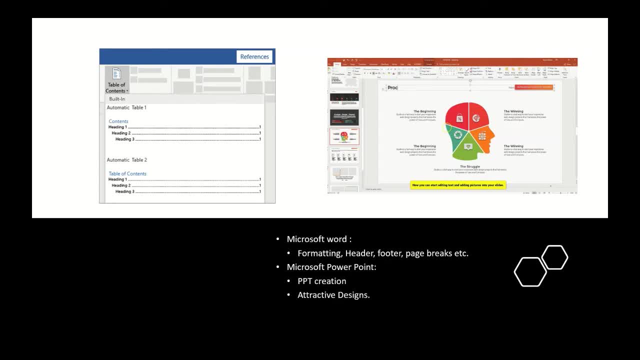 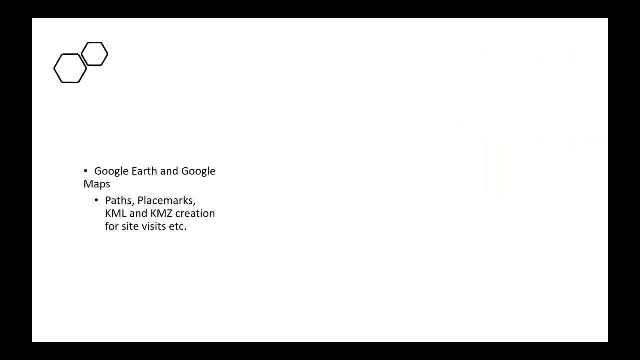 normally this everyone is aware, but some, some more techniques with the linkedin learning and you can learn it from various sources. some useful techniques you can use and make, impress attractive designs and formatting header and footer and page breaks, etc. in a world okay then, yes, google earth and google maps. as i said in the introduction, google earth: 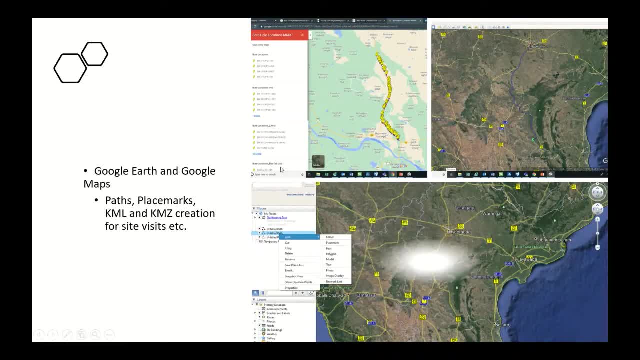 you can see here: google earth from and to destination path. path creation, okay, and then kml, kmz creation for site visits. after that, this place mark and measuring: measuring the distances and measuring the elevation, showing the elevation profile. this especially used for the bypass options. while doing the bypass options, you may use the google earth. so basic understanding means how to 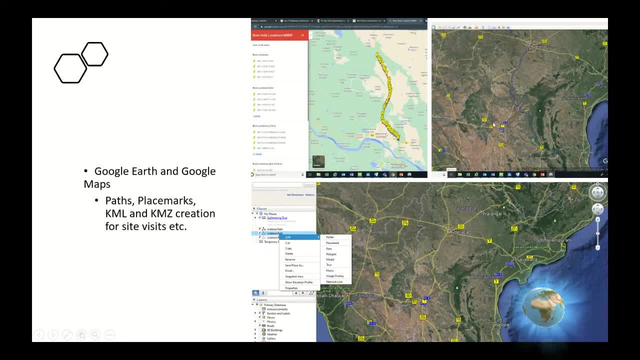 create a pins and all those things you should be aware. okay, and then google maps. one video is there in my channel. you can have a look how to create these pins and how to create their path in a google maps. this will useful for live, live tracking while you are at site. okay, you can. 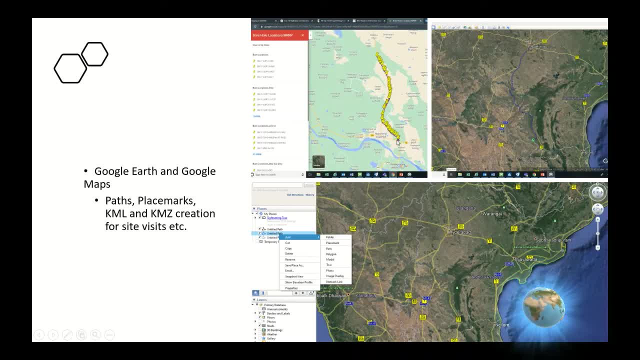 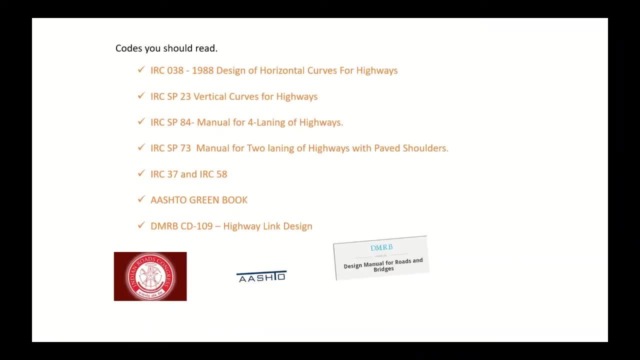 track lively at the uh for that point. okay, so these are the borehole data. okay, that's it, guys. google earth and google maps related information is is uh essential. okay, now codes. i already made a video on that course you should do before starting. highway design: okay. 38 and sb 23, whatever things in the kadialli or. 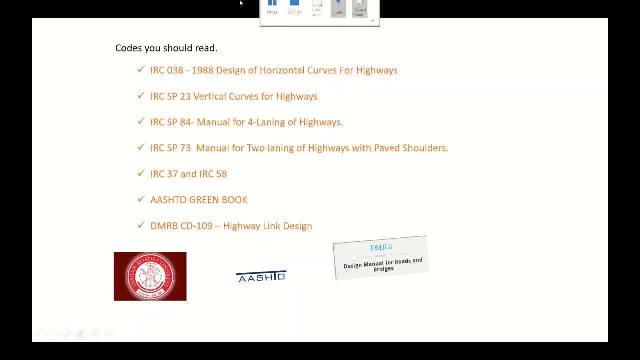 um mentioned. from here. this code should read IRC 38 and SP 23, SP 84, IRC. that is on 58. no need to read everything, just have a overview how the things are made. contents are prepared. okay, that's is enough, actually for pressure. okay, in the engineering service and investigations. this, this is what I said. 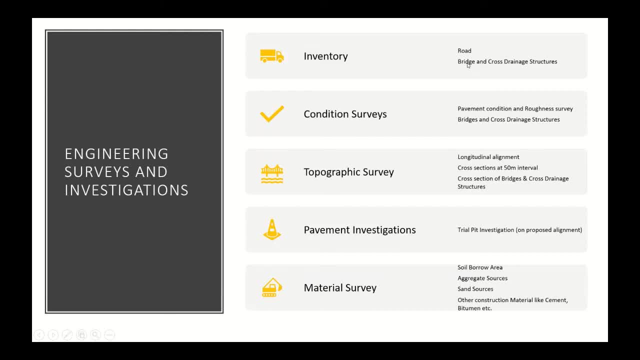 inventory, road inventory, how the elements, road elements without the road and the bridges, all those things. just overview means if you have done a some good project on highway geometric design, so then you must be aware about these inventories. but if you have a just overview also enough, okay, its condition. 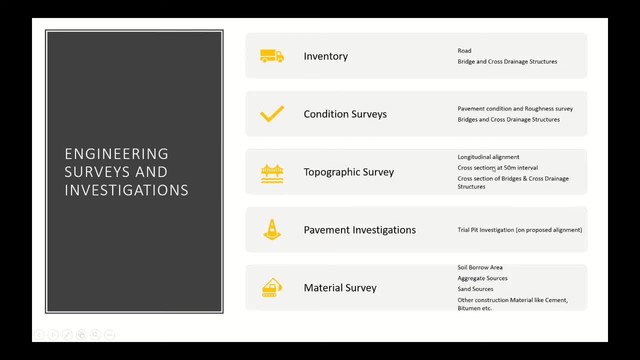 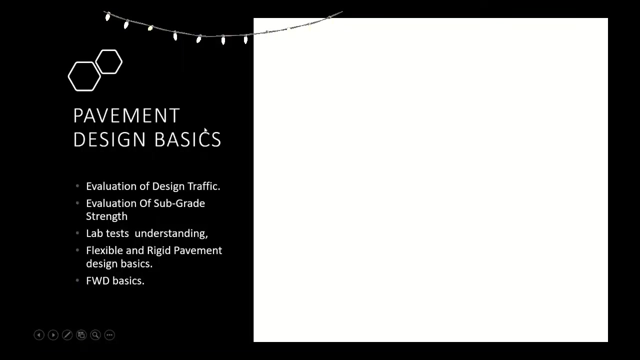 survey: payment condition. topographic survey- our the long section and cross sections point will take payment investigations, trial pit investigations- okay. and then material survey: borrow area, aggregate sources, sand sources, other construction materials, cement and bitumen. these are in depth, but having a worldview that is enough for a fresher, okay. now payment. 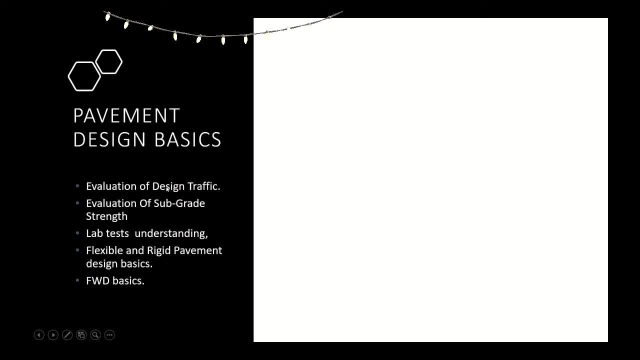 design basics in payment design: design traffic how it could calculated for flexible payment and then for rigid payment. I may say calculation. and then commercial vehicle traffic, okay, and then sub grade stand, CBR value how and lab test understanding how we may use to calculate. so normally in our bachelors